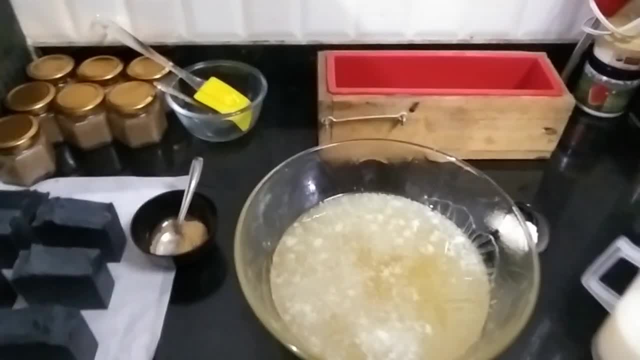 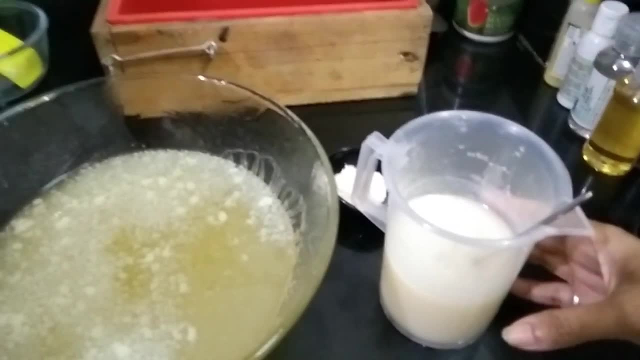 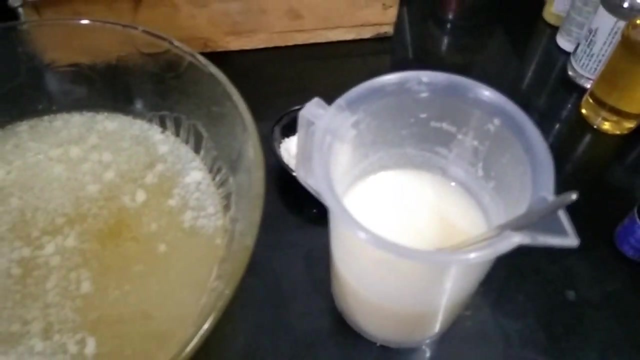 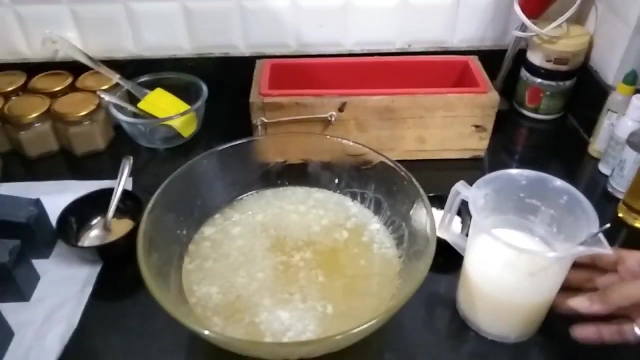 ever is interested to give this soap a try. And here in our lye solution, I have taken milk and lye. We haven't mixed it with water, It's mixed with milk. And for our- you know, the ones who are making cold process soap, who are beginners in making cold process soap- I would like you to watch my video on how we add lye with milk and other liquids. 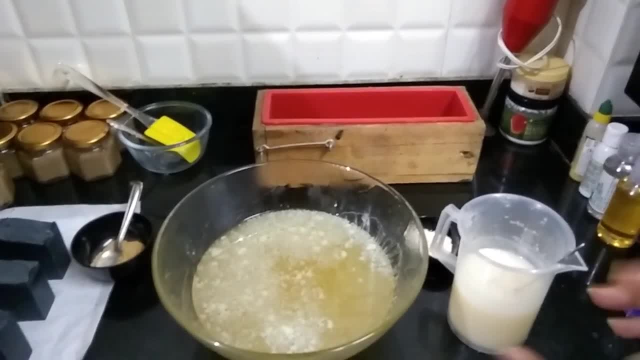 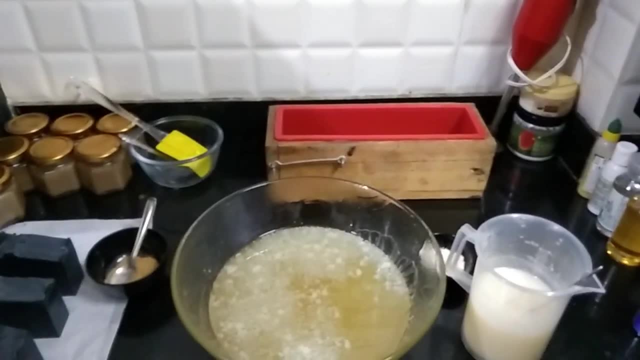 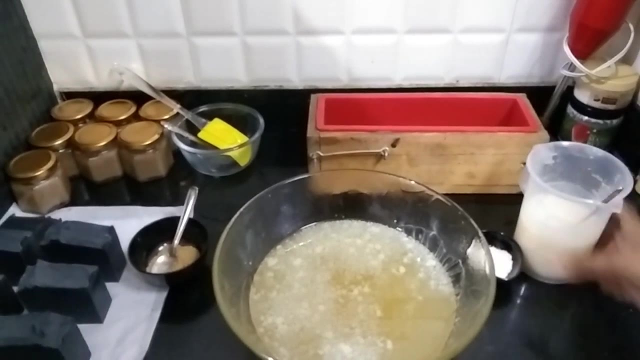 Before you actually start. you know making soaps like these, which contain milk, Since the procedure is a little different from mixing lye with water. So here we have our mixture, our milk and lye mixed together, So we can start with the making of the soap now. 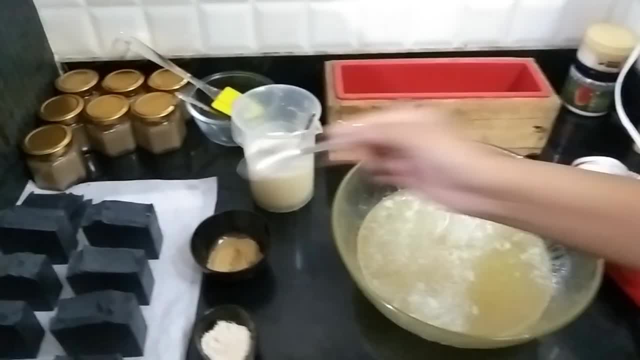 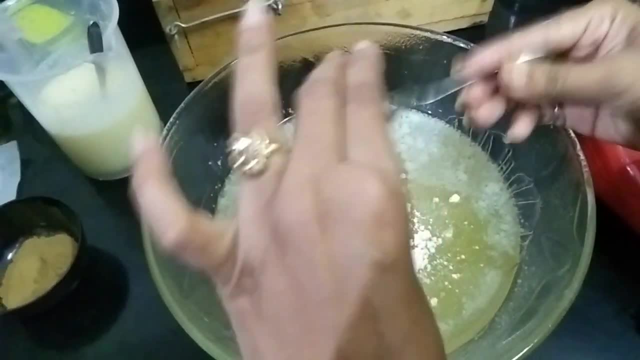 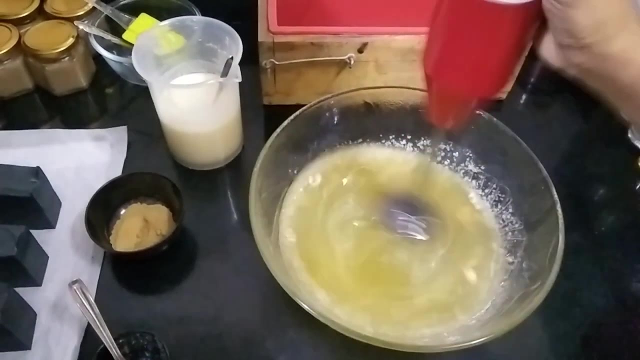 Okay, so here I am going to mix my oats in my oils. Now, oats is extremely moisturizing for the skin. It is basically, you know, a skin softener to keep your skin very soft and supple. So we'll mix this now with the oils. I'll just give it a mix with. 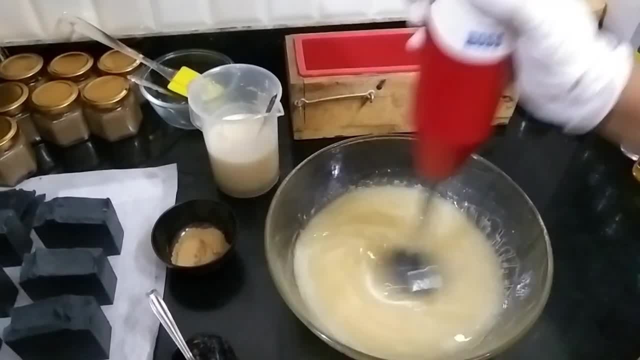 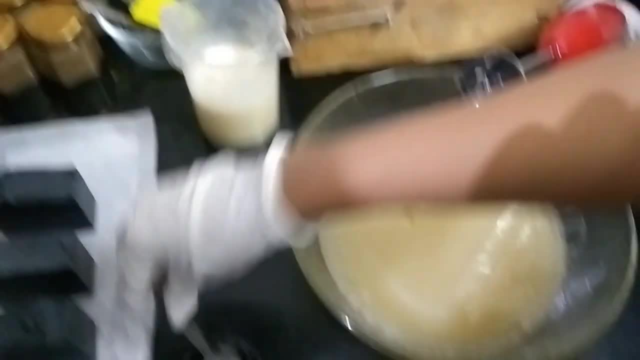 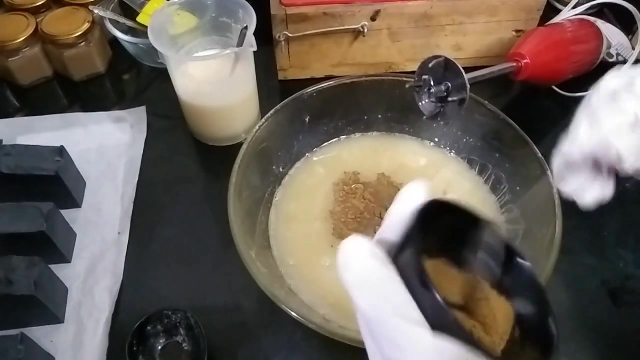 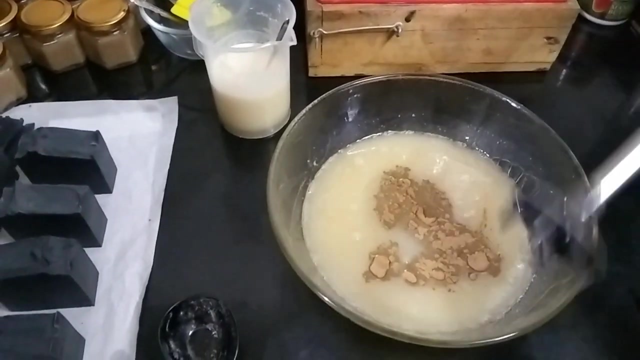 the blender. Okay, so here I have finished mixing my oats in the oils And now I will be mix putting in some bentonite clay. Now, the properties of this bentonite clay is extremely good, for you know, it's like a anti-fungal agent where, if you have any type 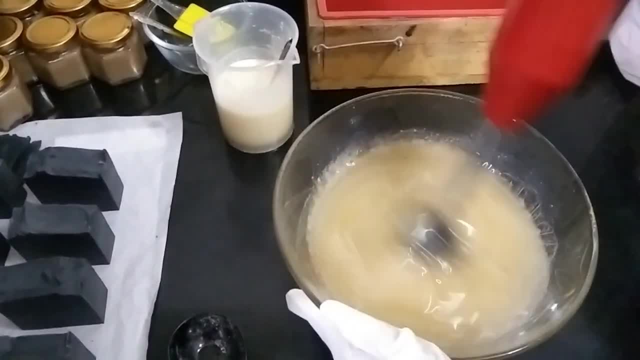 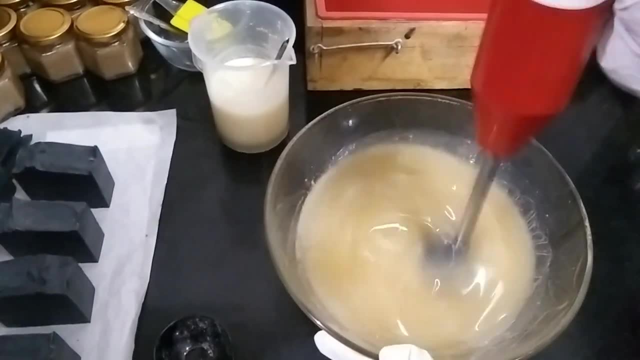 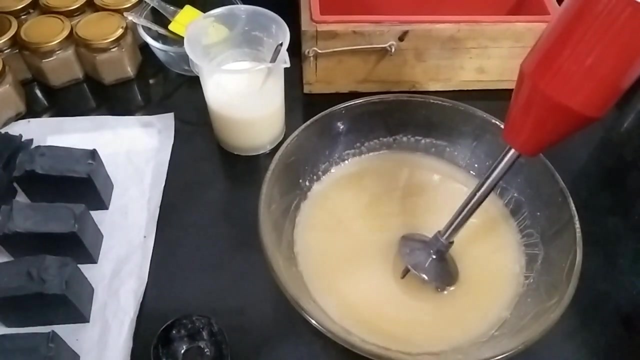 as I said, kids generally tend to get a lot of rashes and all on the skin You know they play out a lot of bacteria fungal infections. So this is extremely good for curing that bentonite clay. You can also check out on Google. you can see the benefits of this clay. 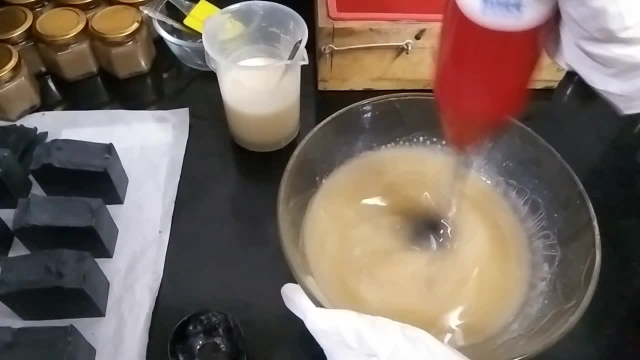 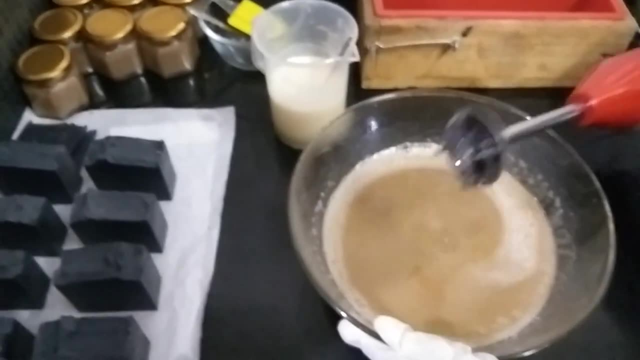 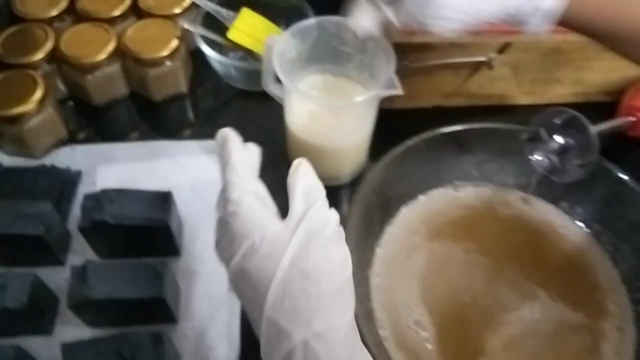 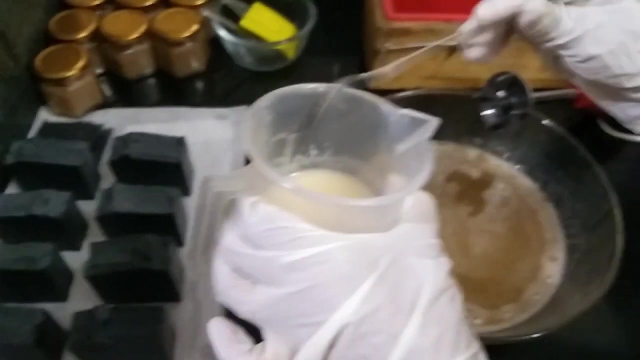 It's extremely, extremely good for the skin, So we'll blend this as well with the oils. Okay, so now I have blended the bentonite clay as well in this, So now it's time to pour our lye into the oils. The lye is cooled down well, So we can add it to the oils. 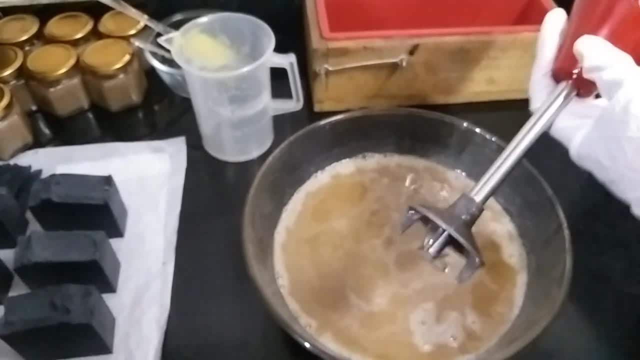 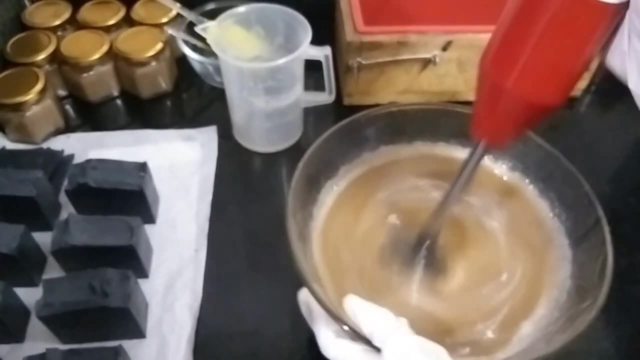 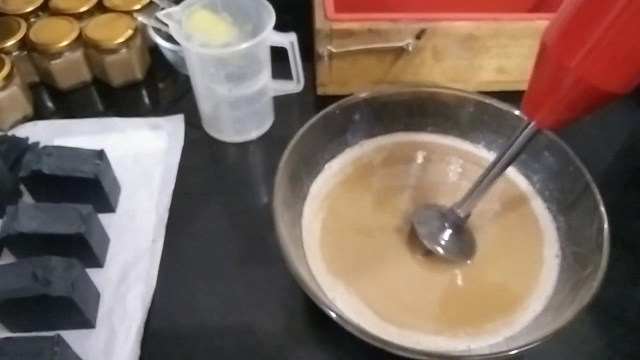 And now we'll blend this till we reach a light trace. Here I'm not adding any type of color or any titanium dioxide to lighten the color, because I want to keep this all natural, since this soap is going to be used by kids, So I don't want to use any other. 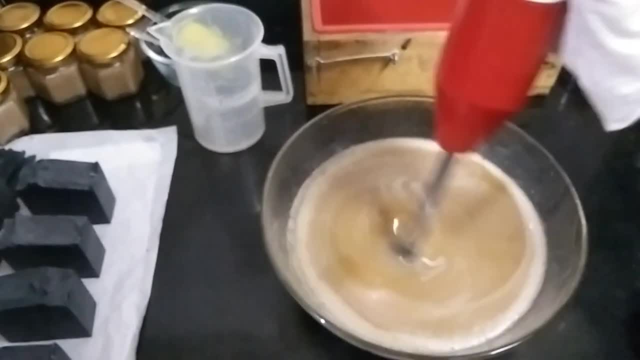 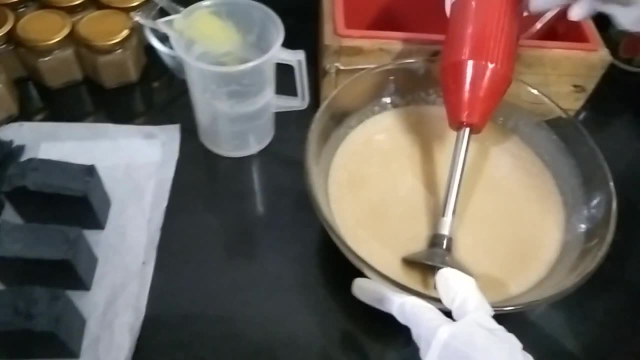 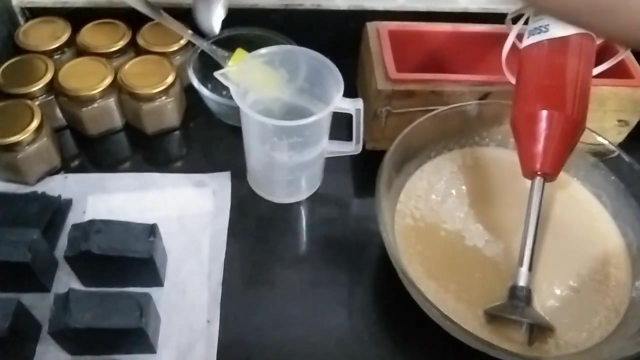 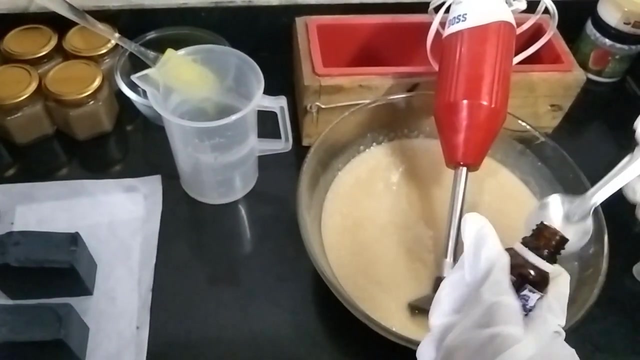 you know, chemicals or anything in the soap. I'm trying to keep it as much natural as I can. Okay, so now I will add my essential oil in this. For the soap, I'm using lavender essential oil, which is again very, very good: a soothing, calming effect. 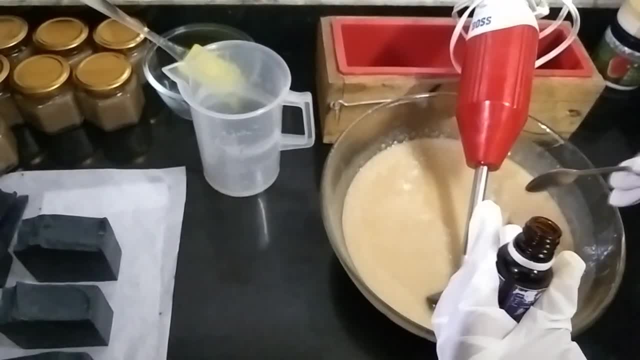 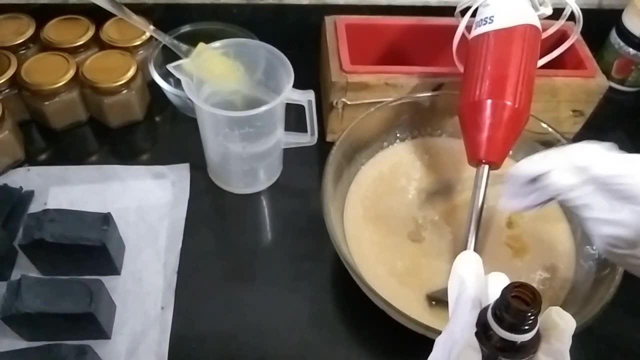 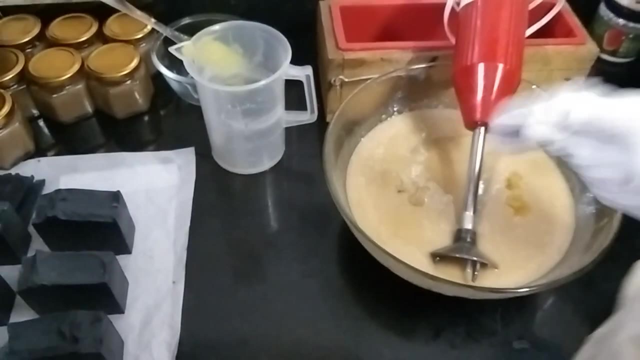 You know the lavender oil gives, and with the calming effect, it is also equally an antibacterial. Okay, You know it has antibacterial properties. So again, which is very good for the skin. So I'll be adding the lavender essential oil for this and I'll just give this a blend. 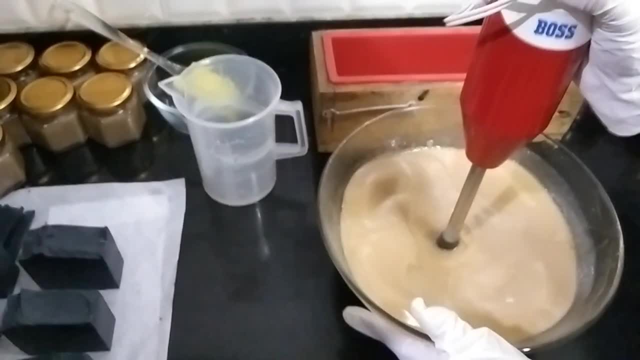 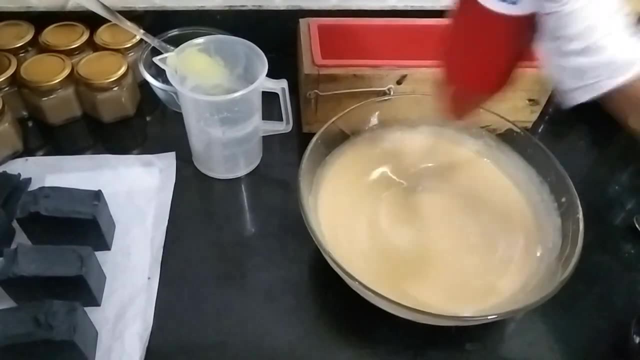 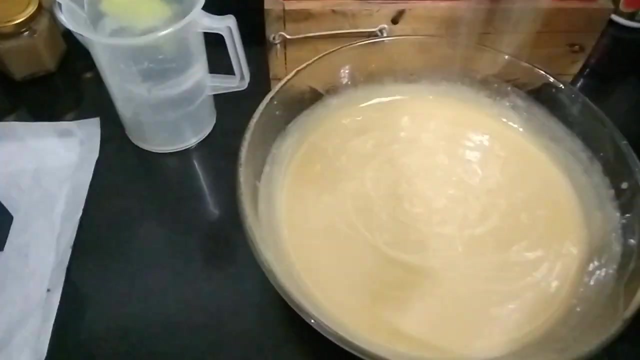 Okay, so now we have already reached trace. For people who don't know what is trace, if you just leave the soap on top and if it leaves a line, you know like a trail type type of a thing, That is how you come to know your soap has reached trace and it's time for you to put 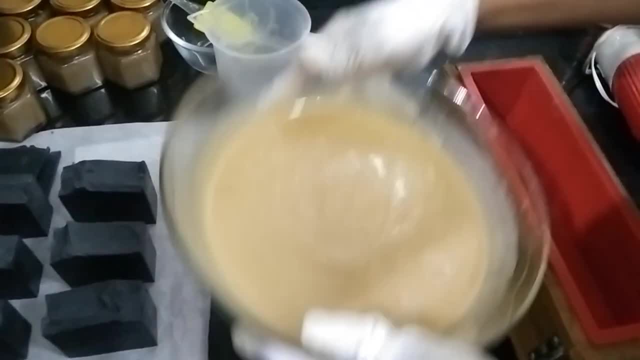 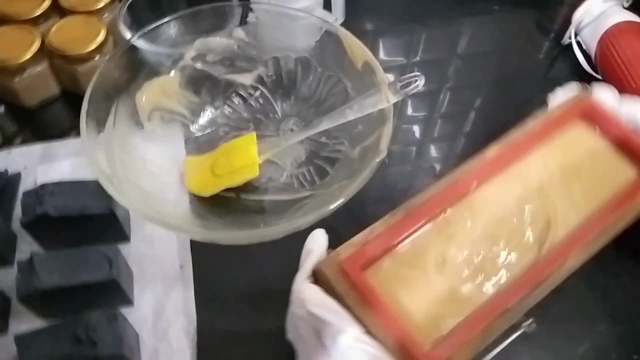 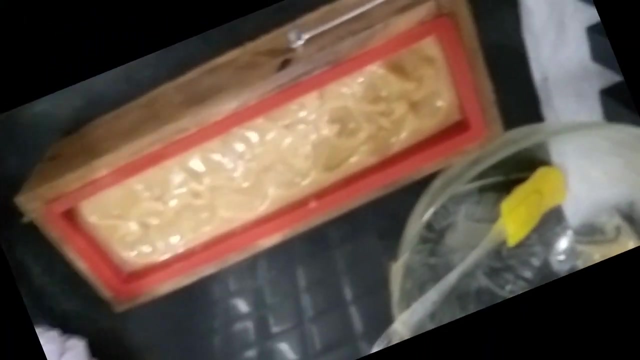 it in the mold. So let us fill up, fill up the soap in the mold now. Okay, we have put the soap in the mold, Okay. so now we have filled up the batter in the mold and I'm just giving it some texture. 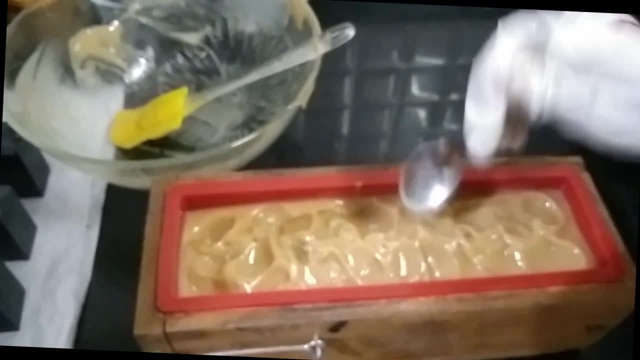 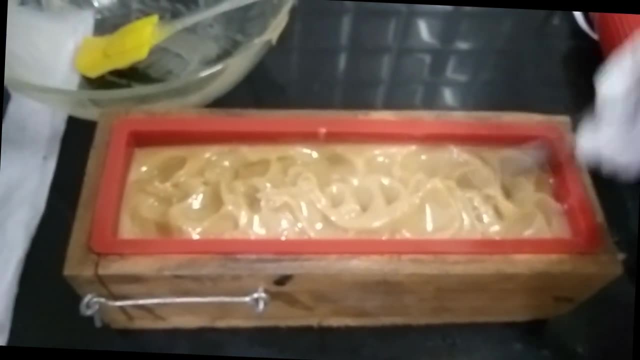 here. If you want, you can add more water. if you want, You can add more water if you want. If you are not interested in texturing your soap, you can just leave it as it is. You can just give it a plain texture. I find texturing the soap makes it look very nice once you. 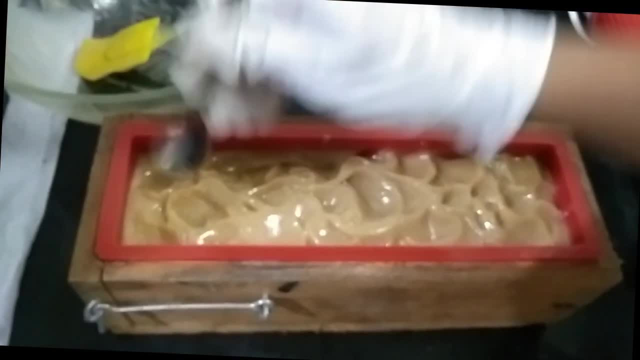 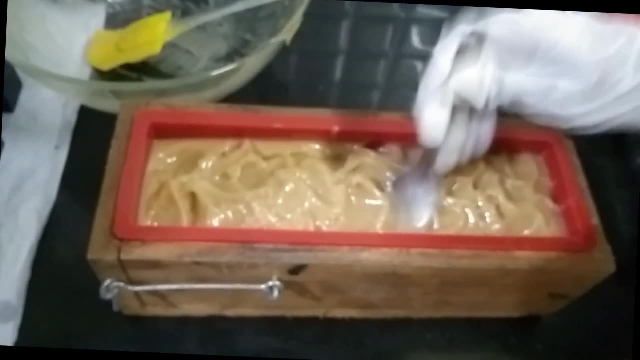 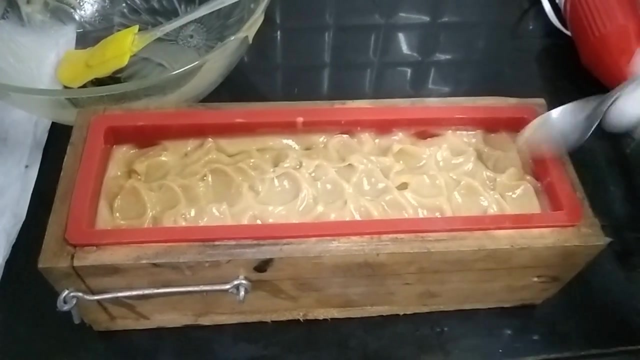 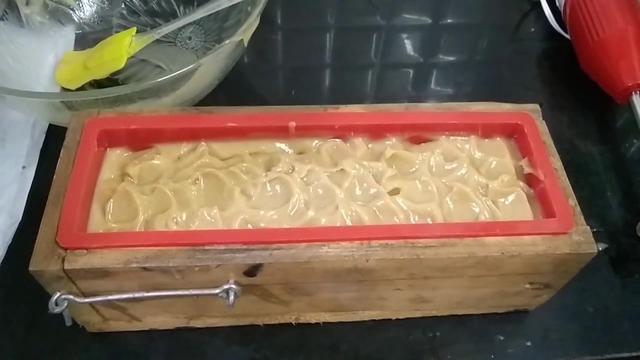 cut the soap. So I'm just giving it some flip flop texture here, Nothing specific, just how I feel. Okay. so I have given this texture here. I'm done with that, Okay. And now we need to keep the soap in the mold for another 18 to 20 hours before we cut the. 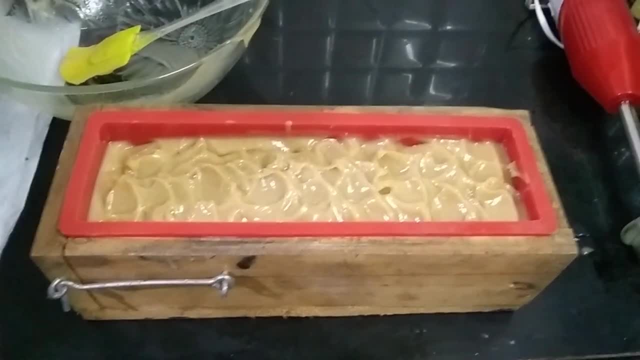 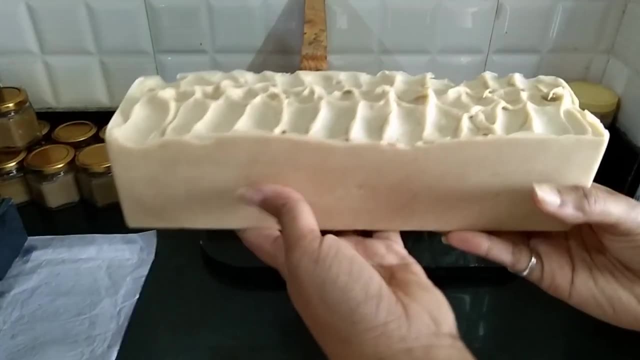 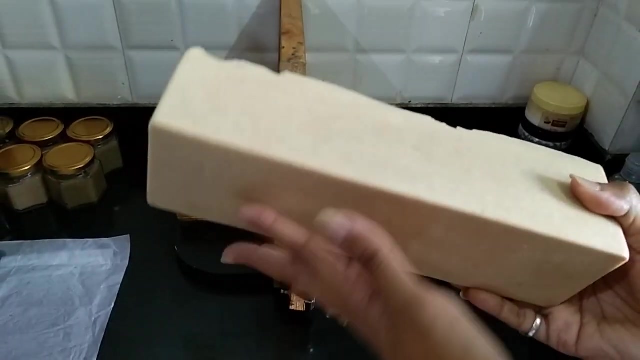 soap. So we will keep it now and I'll be back again when we are doing the cutting of the soap. Okay, so now we have unmolded the soap. It's been about 20 hours, I guess 18 to 20 hours. 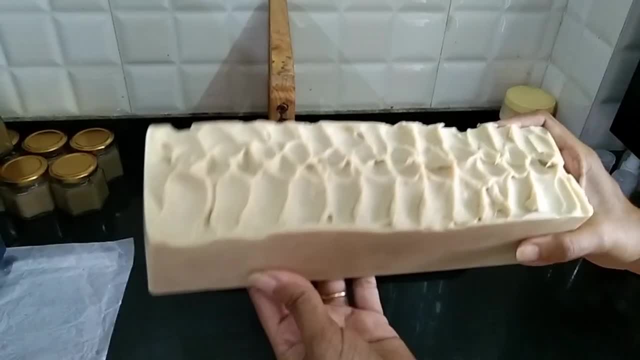 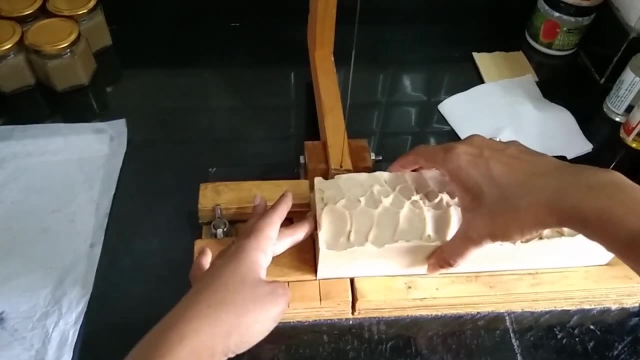 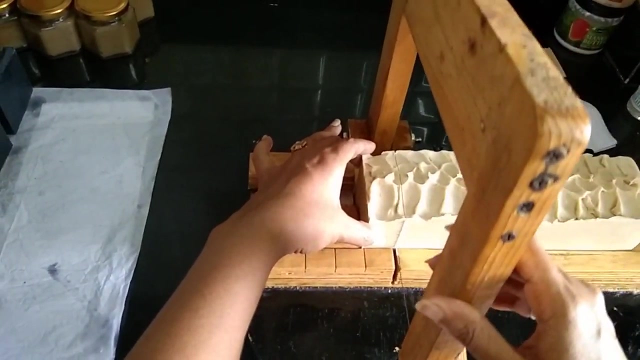 and it's done. It's hardened up very nicely. So now we'll just start with the cutting. I'll just show you how we do that. I hope you all can hear that noise that just came. I don't know, it just started happening. 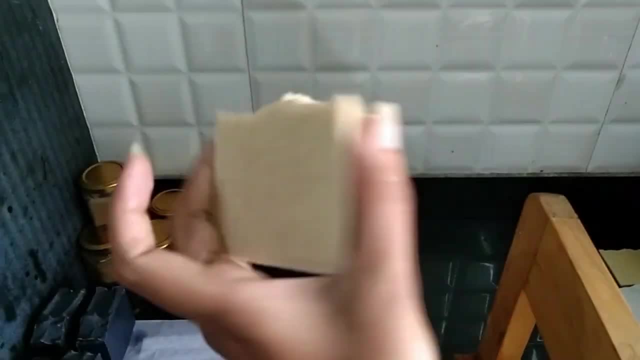 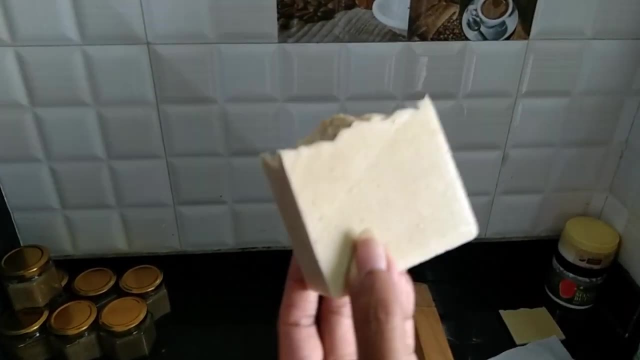 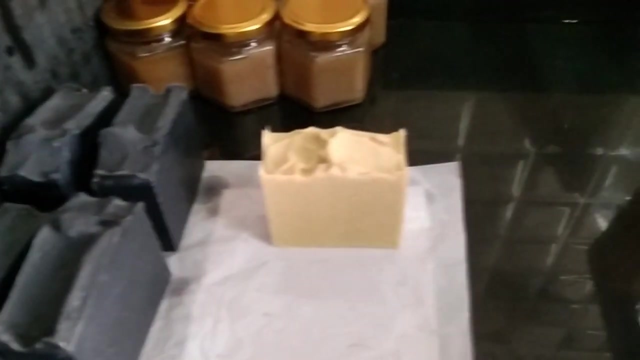 All right. so this is how our milk and oat soap looks from the inside. It's gelled very well. You know It's got a nice color. Yesterday when we had put it in the mold, it was a little darker in shade, if you see, But I think once it's dried it's got this nice light cream color. 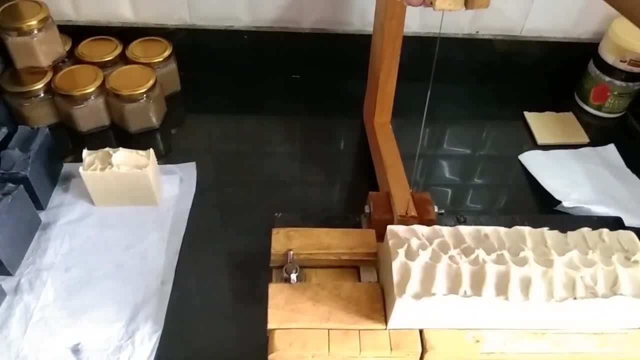 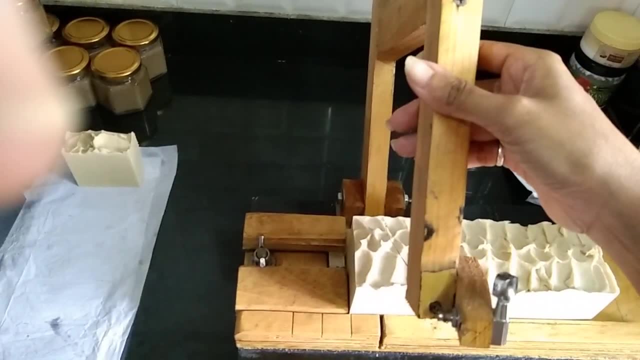 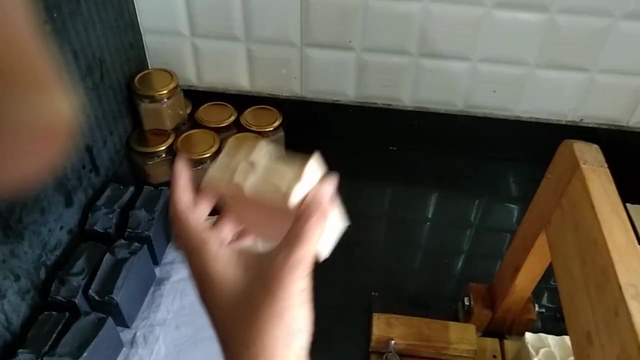 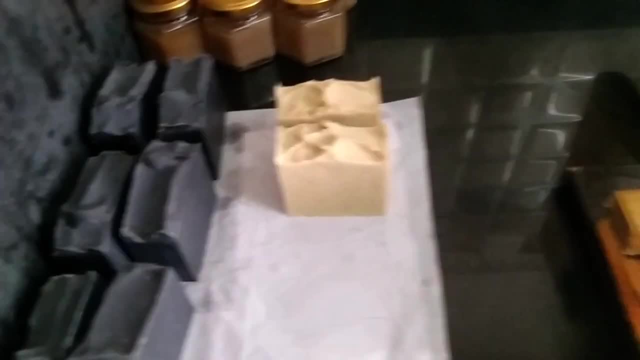 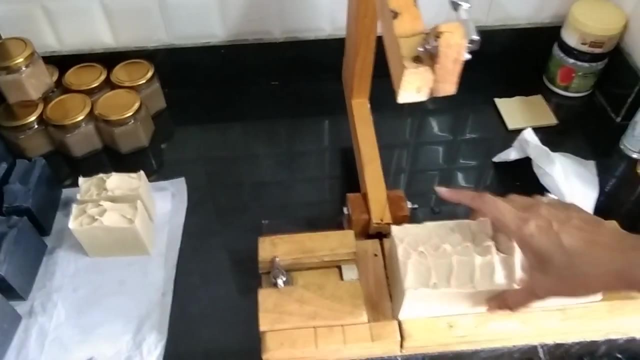 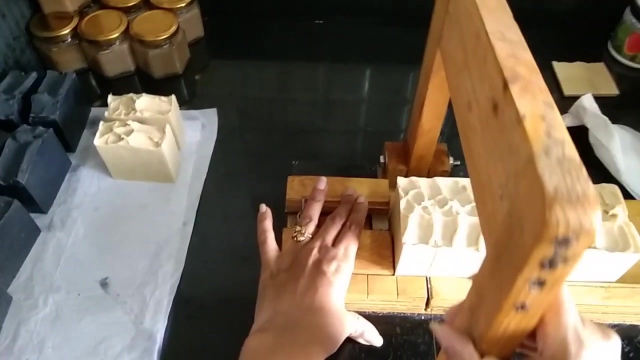 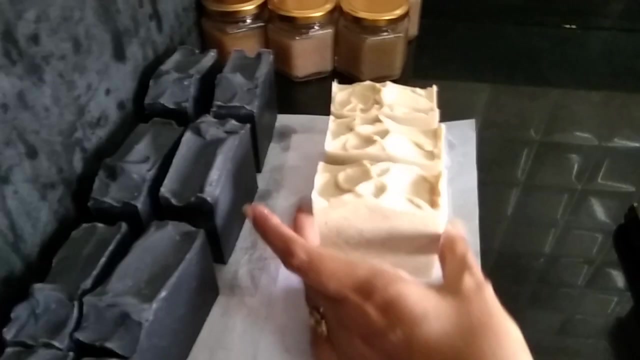